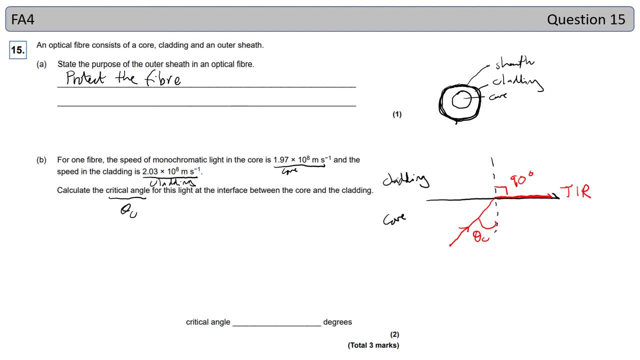 where the angle of refraction is 90 degrees. So we know from Snell's law that n1 sine theta 1, where n1 would be the refractive index of the core, is equal to n2 sine theta 2, where n2 is the refractive index of my cladding. 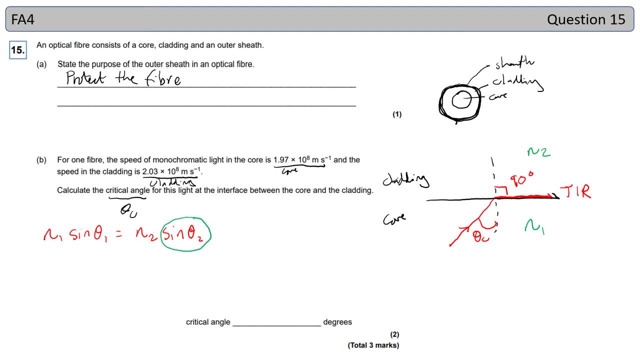 Well, sine of Theta2 becomes sine of 90, which just becomes one. So I can rearrange this to say: okay, therefore, sine equal to N2 over n1.. Okay, therefore, sine of the critical angle is equal to n2 over n1.. 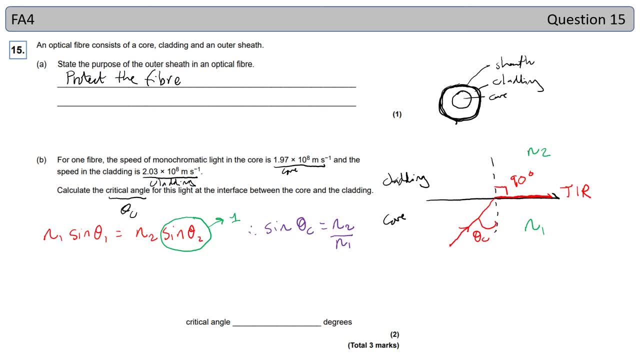 But that means I do need to work out the refractive indices of each of these. Well refractive index is speed at criptoplanet level, which is Earth's airport. Well refractive index is N2 over N1.. Well refractive index is speed at Vorskel. Well refractive index is speed at volumetricının viviridez ground mu. but that means I do need to work out the refractive indices of each of these. Well refractive index is speed at arrival at 9 and at G. Well refractive index is speed at release of delivery at the movement balance andmoon to birth. 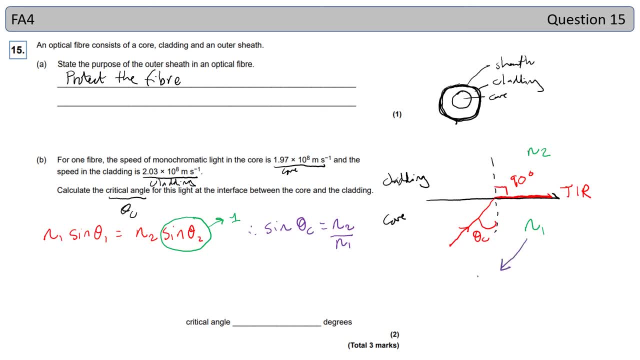 Well, refractive index is speed of light in a vacuum over speed of light in the material. So for N1, which is our core, that's this one here. So that'll be 3 times 10 to the 8.. Remember, our refractive index always has to be above 1,. 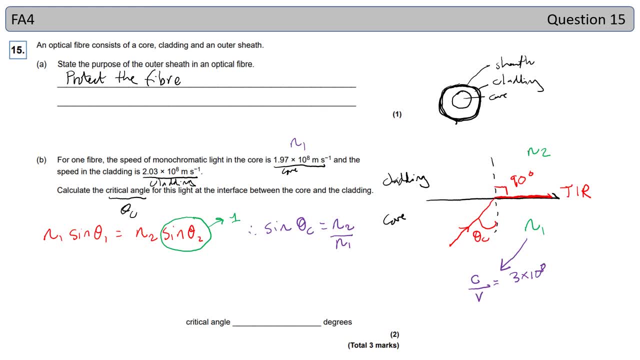 and it's a ratio of the speed of light in a vacuum to the speed of light in the material. So for N1, it's 3 times 10 to the 8, over 1.97 times 10 to the 8.. 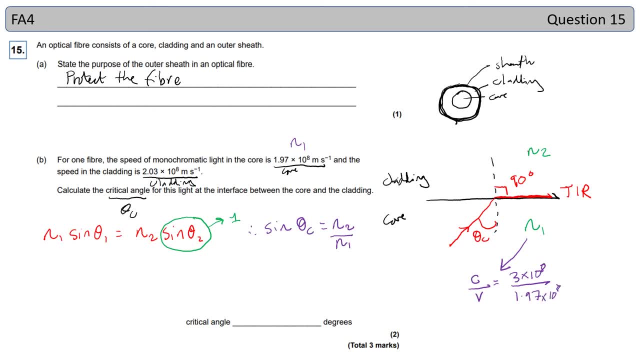 And that gives us a refractive index of 1.52.. Remember, there's no units on refractive index, It's just a ratio. And then for N2, same again: C over V is equal to 3 times 10, to the 8 over 2.03.. 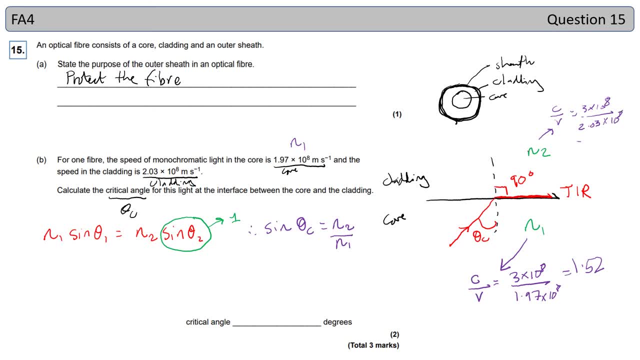 Times 10 to the 8. And that gives us a refractive index of 1.48.. So once I've got my two refractive indices here and check that makes sense, for total internal reflection to occur I must be going from more optically dense to less optically dense.